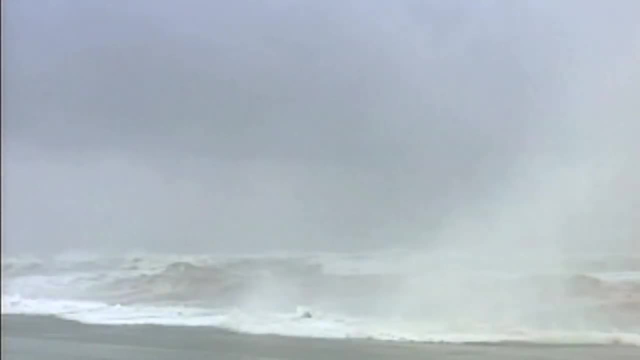 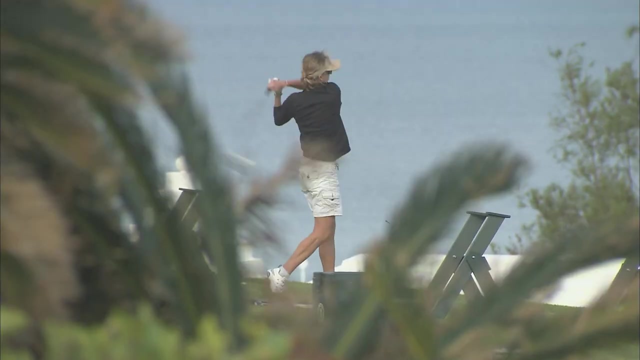 that lends a huge amount of energy to hurricanes and tropical cyclones. Dr Tony Knapp is the director of the Bermuda Institute of Ocean Sciences, or BIOS. Famous for its luxurious golf courses and pink sand beaches, Bermuda is also home to one of the world's leading 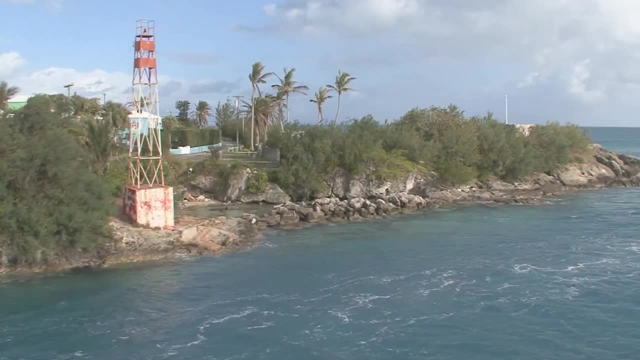 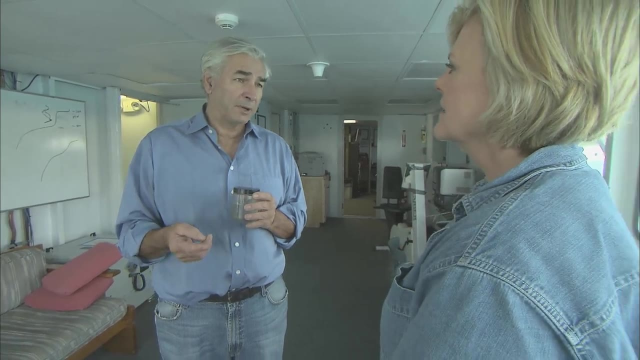 institutes for ocean studies, with a focus on water temperatures. Here off Bermuda we have probably a better view of it than many other people are going to have over time. Bermuda is located over 600 miles, or almost 1,000 kilometers. 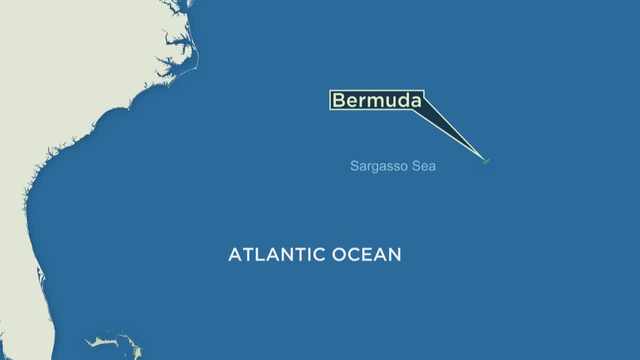 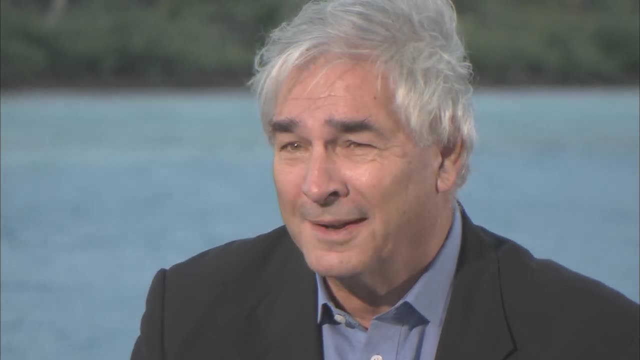 from the coast of North Carolina in an area of the Atlantic Ocean called the Sargasso Sea. We like to think of the Sargasso Sea in the North Atlantic as the canary in the coal mine. It's the smallest ocean, It's between North America and Europe And we think, if we're going to see 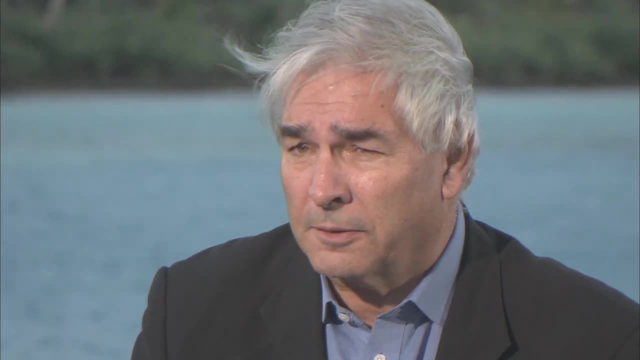 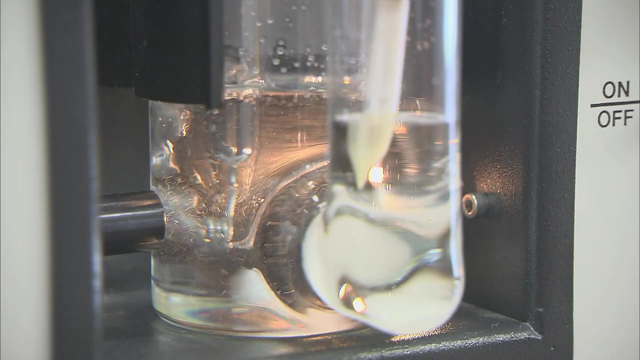 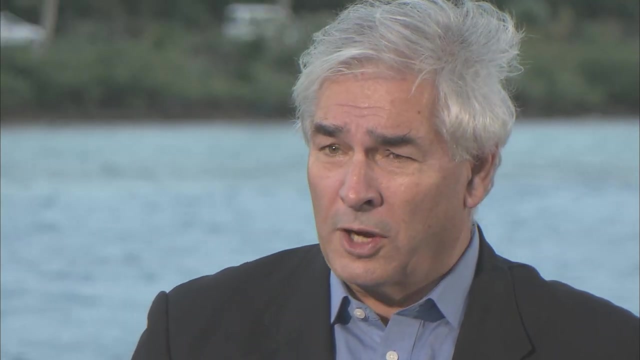 changes. we'll see them first here in the ocean off Bermuda. Scientists at BIOS have been measuring the temperature of the ocean since 1954, making it one of the world's longest ongoing studies of ocean data. Well, you measure the temperature of the ocean in many ways. In the old days you used to do it with buckets and thermometers. 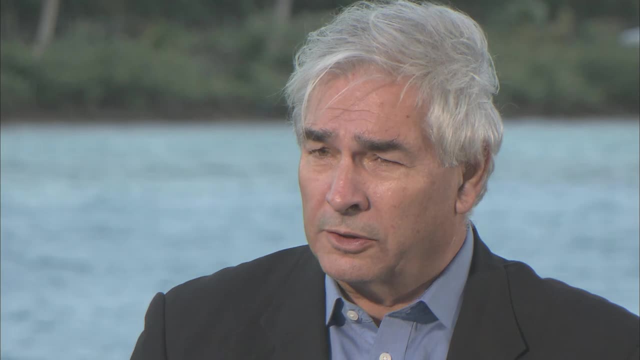 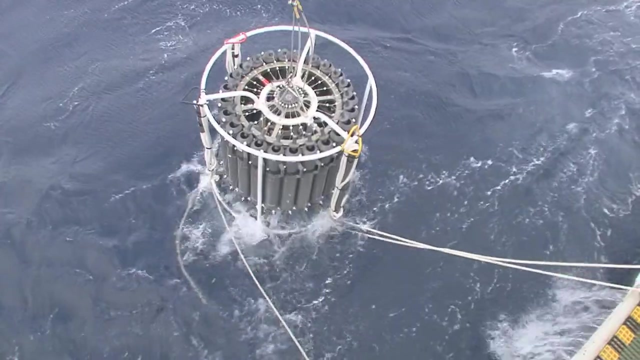 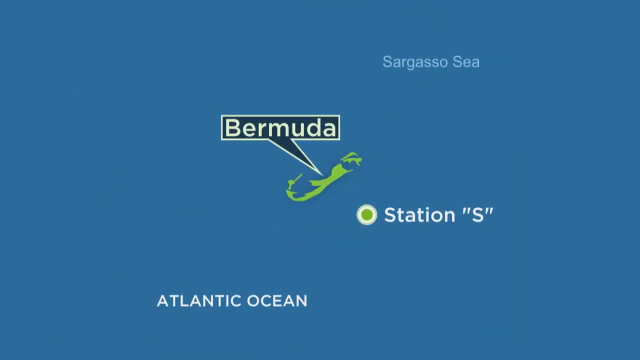 Now you use sophisticated instruments called conductivity temperature and depth recorders. These recorders, called CTDs, are large measuring instruments lowered deep into the water at specific locations in the ocean. On this day, Nap and his team are headed to Station S. 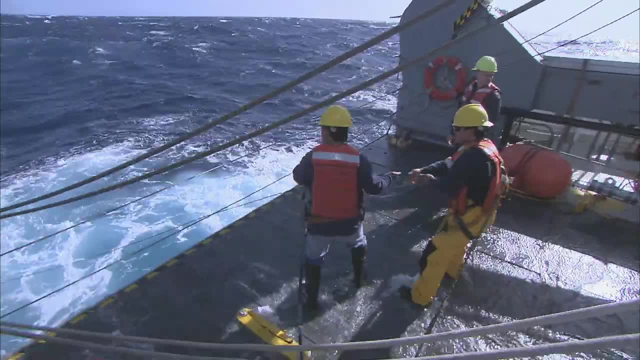 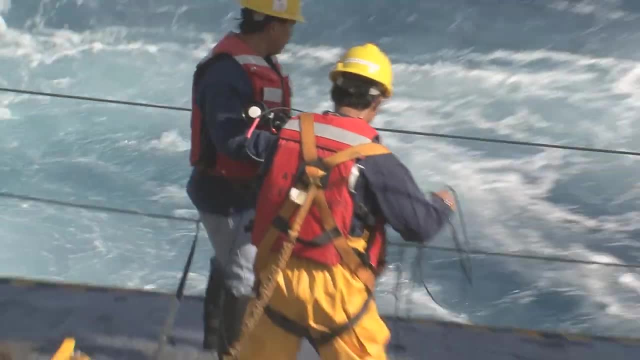 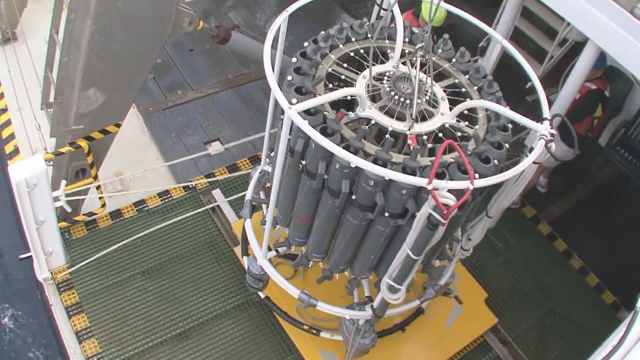 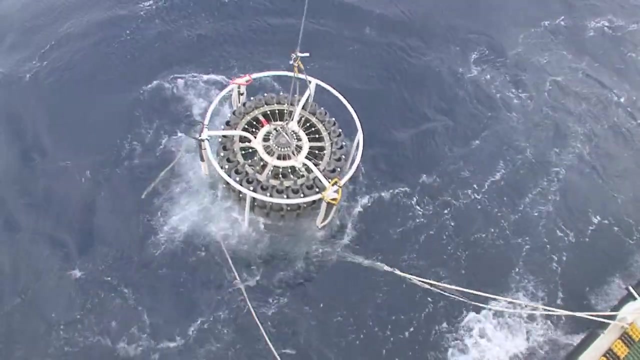 The weather is not going to be our friend today, unfortunately. The wind's out of the west, It's 35 to 40, and some higher gusts. The seas are anywhere from 14 to 16 feet or higher, Lowered to a depth of 3 kilometers or just under 2 miles. the CTD records temperature, salinity, carbon dioxide levels and captures water samples. 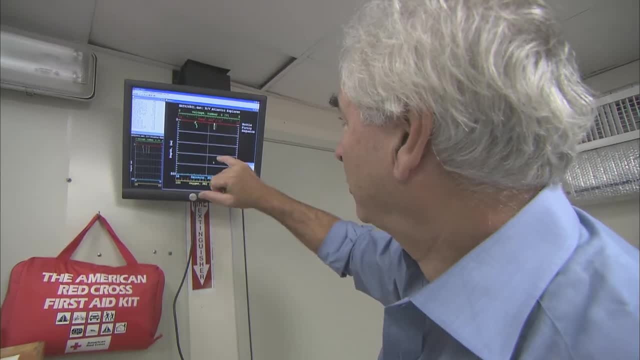 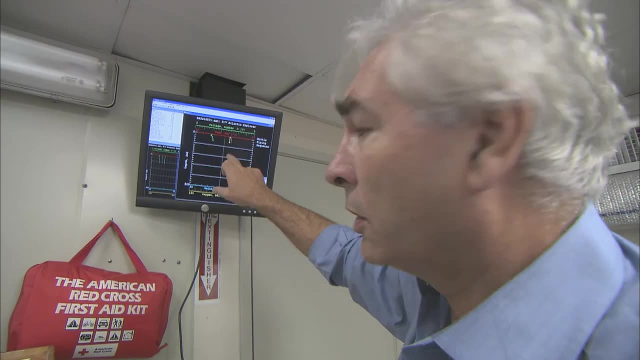 This is a screen for the output on the CTD. The temperature will be in red. Blue is salinity, The salinity is the saltiness and yellow is the oxygen content At BIOS. all of the data is then carefully logged and analyzed. 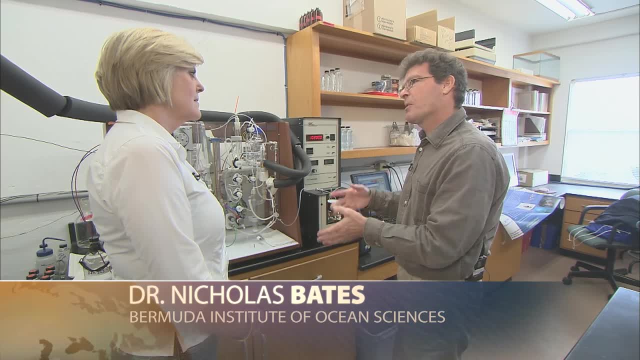 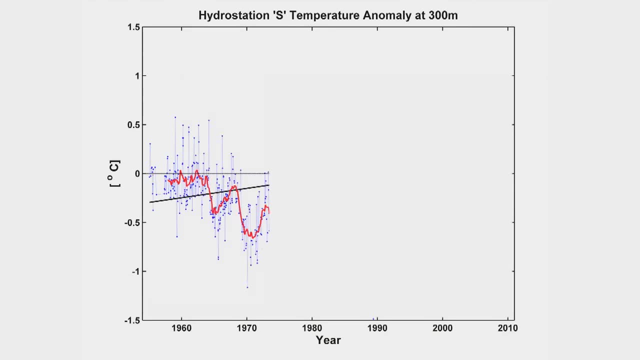 With this instrument, we can see changes that happen over the season, over the year and then from year to year. Using ocean temperature data going back several decades, BIOS research can trace the warming trend. In the past 56 years it has risen half a degree Celsius. 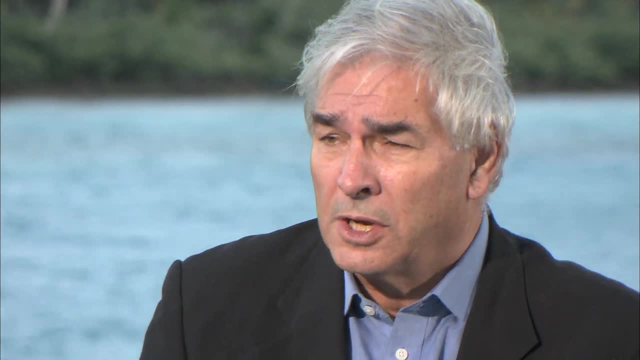 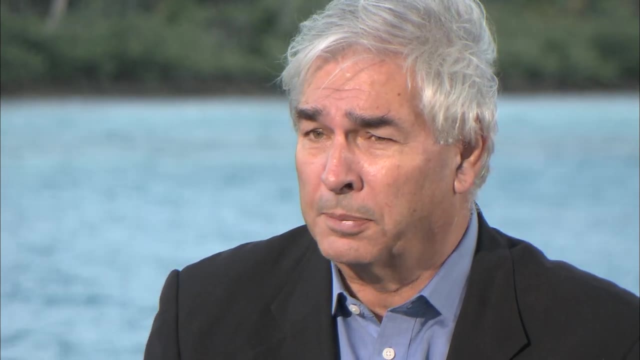 Since 1954, we've seen, on average, the temperature increasing by a small amount, but equivalent to what is really a half a watt per year, which doesn't seem like a lot, but over the whole of the ocean it's a lot. 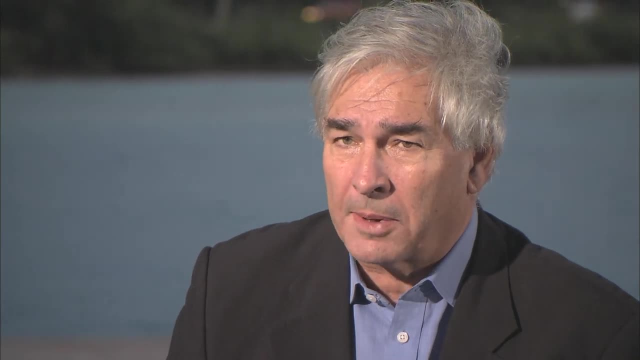 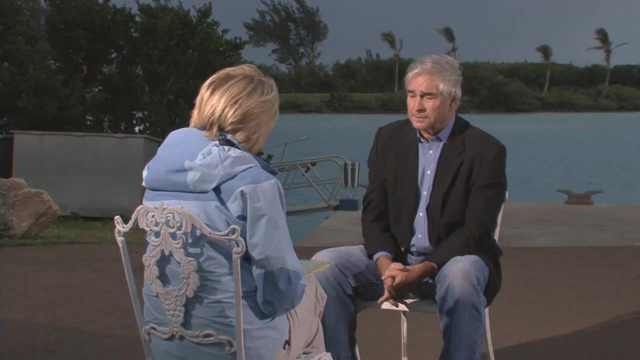 What's? a half a watt? It's not much. It's about a hundredth of a degree per year. It's not a lot, But that small of a difference can have a huge impact. Yeah, Really, Yeah, Yeah, because it's going on every year. 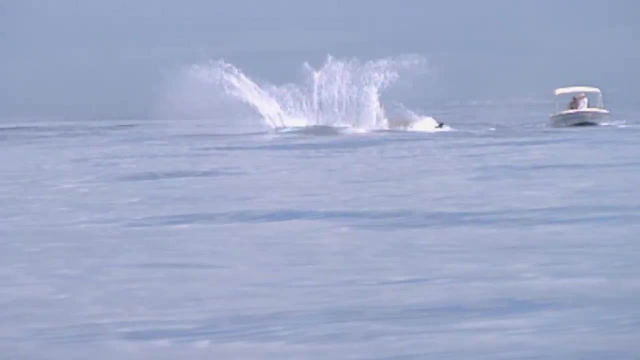 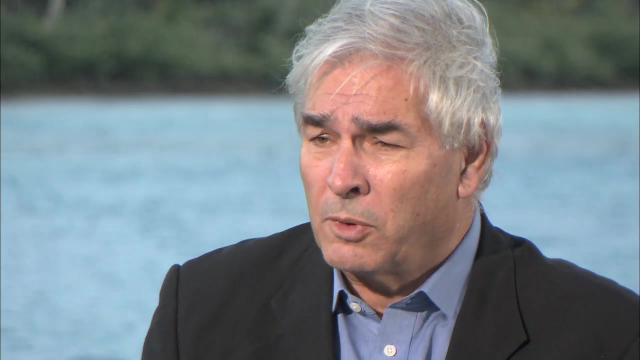 You think about how big the ocean is and how deep it is and how much energy it has. I mean, it's a tremendous source of heat. Where is that warming coming from? Well, the warming, we believe is due to changes in CO2 in the atmosphere. 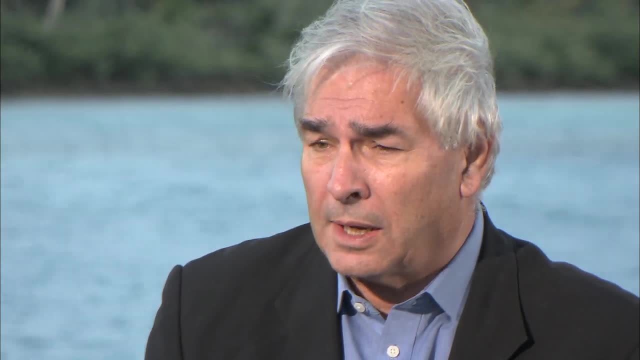 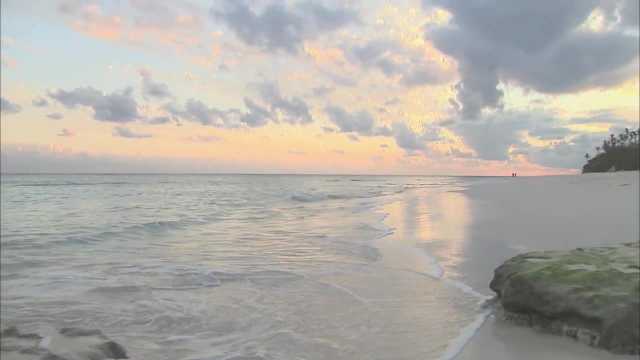 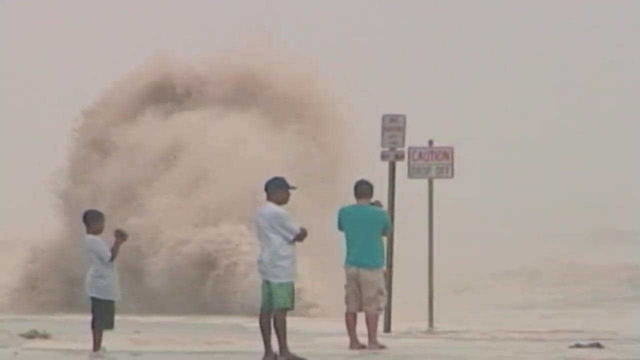 the atmosphere getting warmer and the surface of the ocean getting warmer, And that transfer of heat is being made into the ocean. So what is the impact of a warmer ocean? The increasing temperature causes the ocean to expand and raises sea levels. The tide's going up by 3.2 millimeters a year. 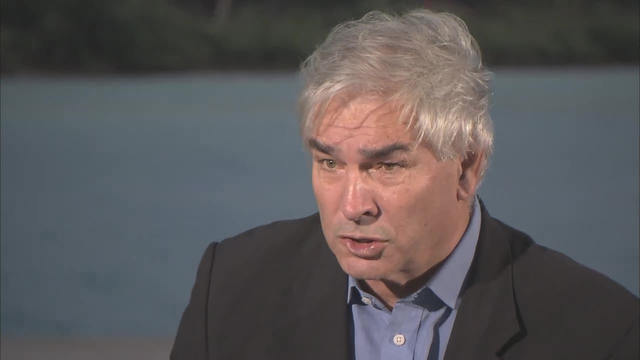 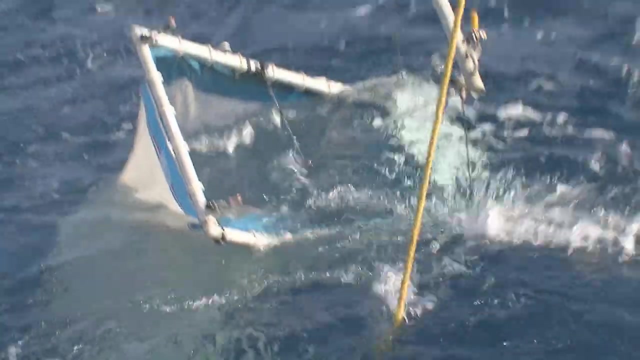 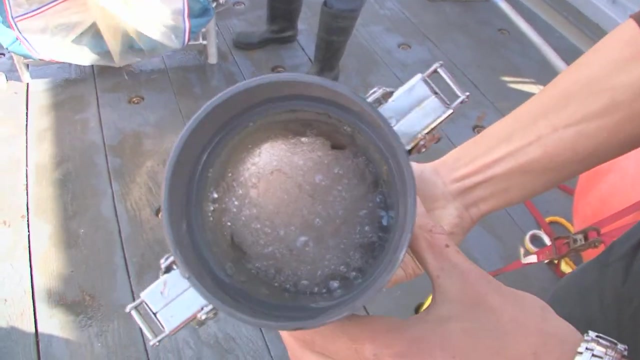 Half of that is attributed to the ocean warming down to 700 meters. The ocean's, on average, 4,000 meters deep, so it has a lot more to expand. Warming temperatures can also impact the growth rates of certain organisms at the very bottom of the ocean food chain, like phytoplankton. 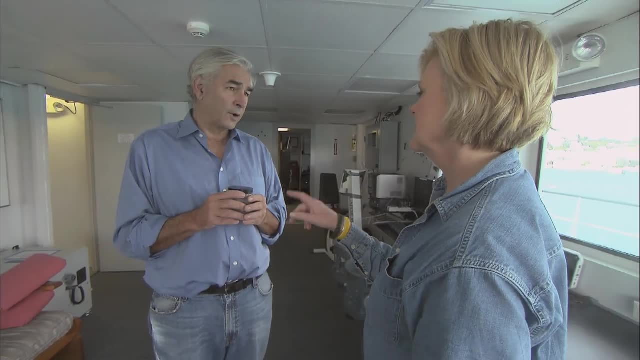 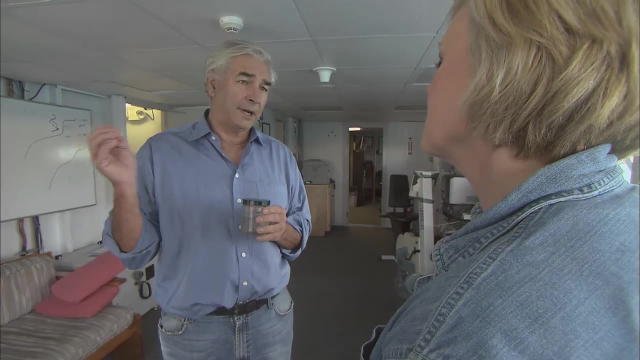 And so if you see changes in phytoplankton, does that mean that we are going to see changes in the food chain of the ocean? If the organisms that eat those organisms, like plankton, for example, can't eat those plankton, then yes, you'll see changes. 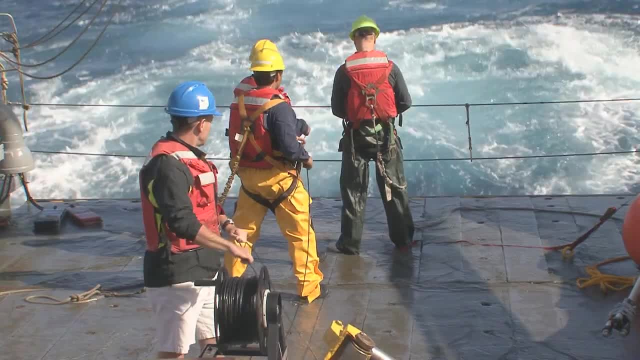 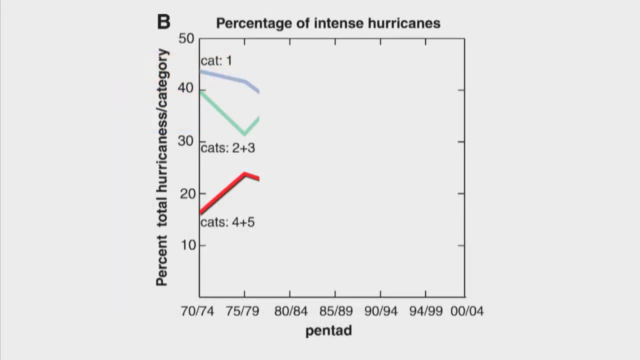 And the small changes being recorded could bring even stronger storms. This report, published in 2005 in Science Magazine, shows the gradual rise of the number of Category 4 and 5 hurricanes over recent years, An increase in stormwater and a rise in sea temperature.